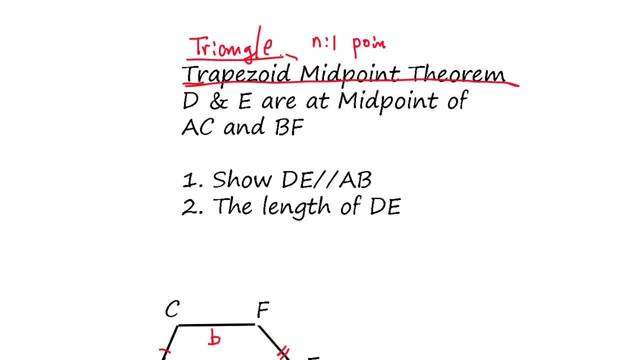 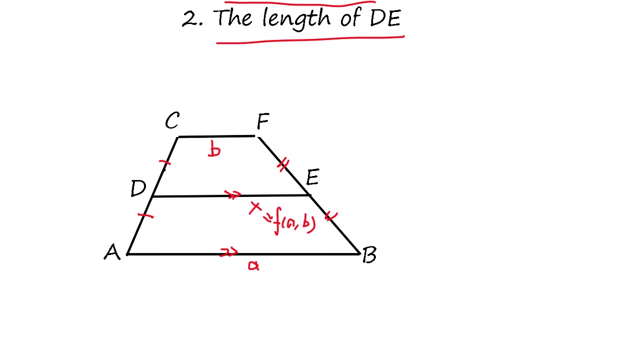 into one point theorem And this one in another video. we went through this theorem. We use the same method to prove this two point here for trapezoid. So how do we do that It's not triangle? Well, what we do is we extend this line and make it triangle. Okay, 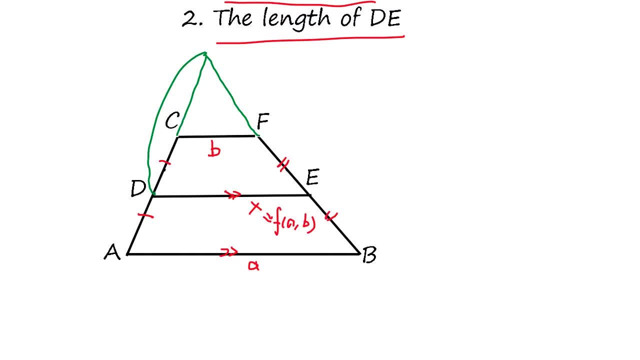 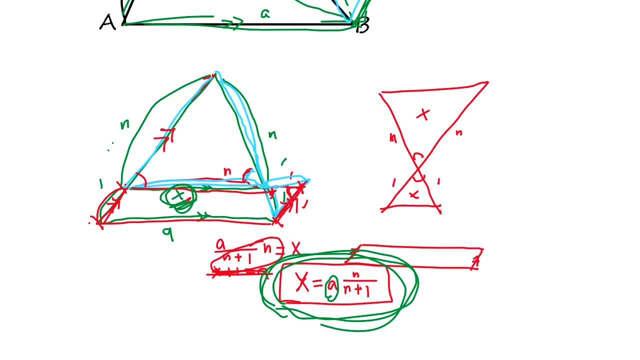 So if we know this is n to one, then we know the answer already In the previous video: x is n to one, Okay, Okay, So we'll see the answer right. So x is n to one, Okay, So this is a times n over n plus one. 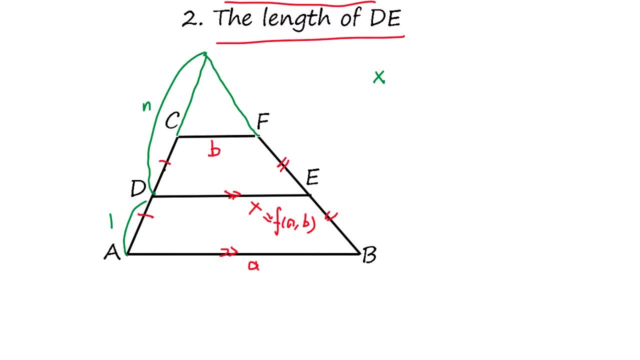 Right, So x equals a n over n plus one. We know this answer already. The question is: how do you get no? ah, how do you get n? Okay, so we use triangle n to one point theorem again for this guy. Say: you have x is n to. 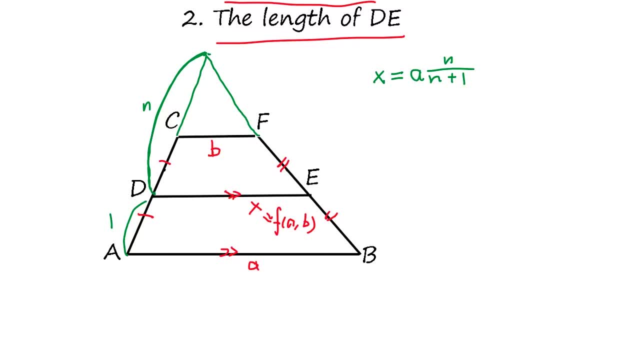 one, then you get a n over n plus one. Okay, Okay, So now we'll do the previous one. now, Okay, Okay, say it's N. So if that's N, we have to extend this to make same way the two similar triangles. 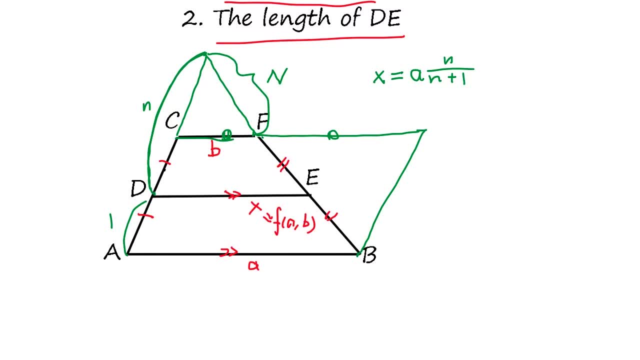 So the ratio of this N to 1, how much you have to extend? So how much do we extend this part? Well, the relationship will be same: B equals AN plus 1 over N. OK, OK, OK, The same equation. 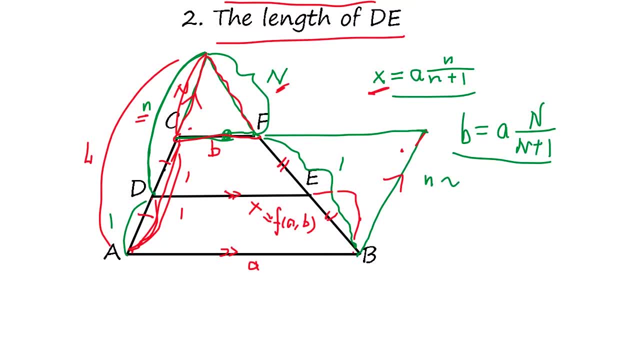 Now we have to get the relationship between this and N. How do we determine that? Suppose this entire length is L, right, OK, And this is N, and this is 1.. Well, this length is twice as long as this one. 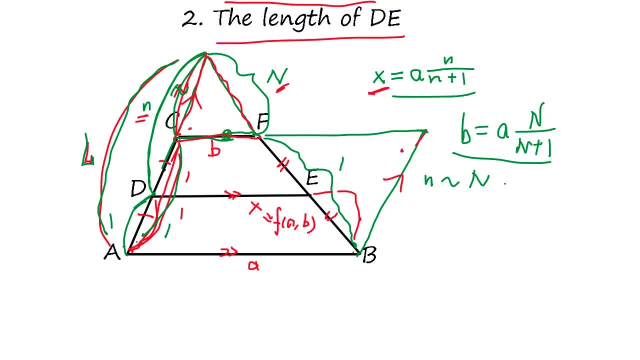 But this length is going to be N plus 1 over L Right And we twice that, which is this is equal to N plus 1 over L. So 2N plus 1 equals N plus 1.. So N equals 2N. 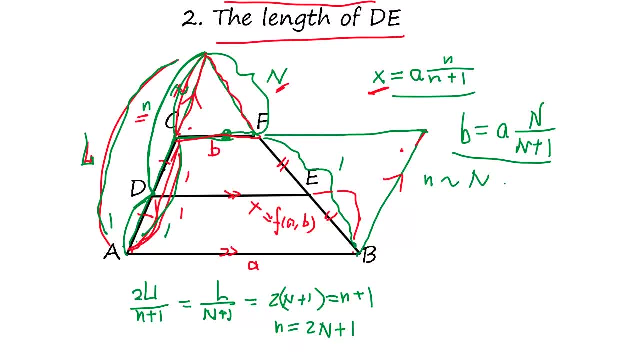 Right, So we plug this in here. we get B equals A. Well, actually we have to do this. N equals N minus 1 over 2.. We plug this one, We plug this one into here. So N minus 1, 2, N minus 1,, 2 plus 1, multiply 2.. 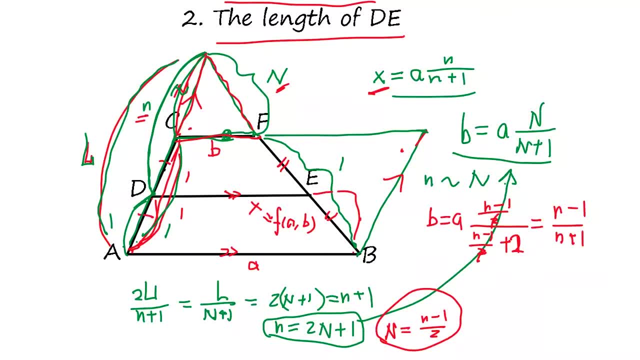 So N minus 1, N plus 1.. OK, So that's the relationship. B equals A, N minus 1, and N plus 1.. So we get N from here. So B minus A, we say temporary C. The C equals N minus 1, N plus 1.. 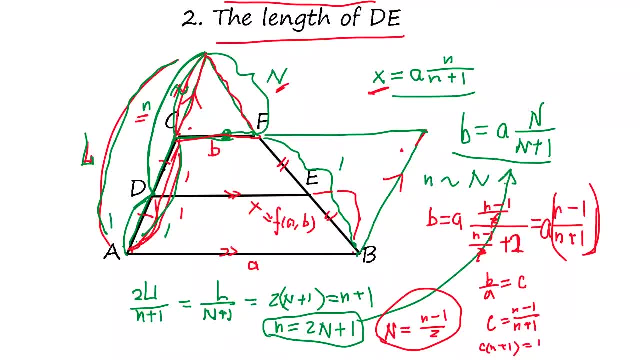 So C N plus 1 equals N minus 1.. So what happened? is N 1 minus C equals C plus 1.. So N equals 1 minus C. OK, OK, So N minus 1 plus C plus C plus 1.. 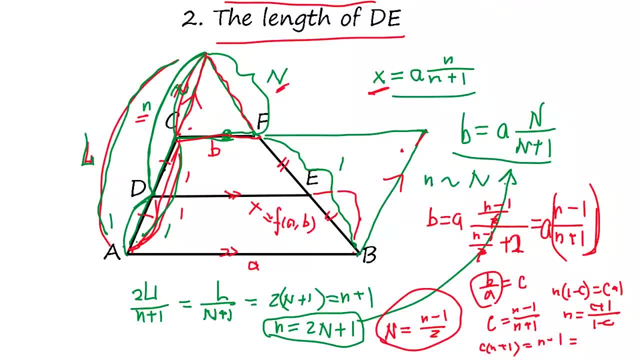 C is this: So multiply A, both A minus B, A plus B, So N is A plus B over A minus B. We plug in that Then A A plus B, A plus B plus A minus B, OK, OK. 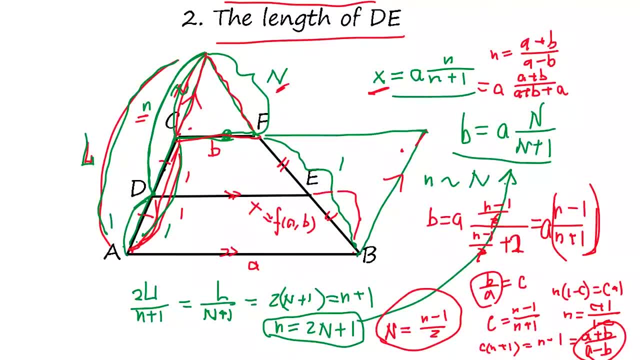 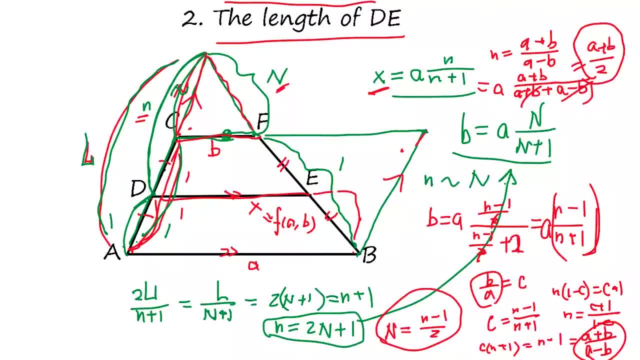 OK, I hope you enjoyed this video and if you, please check out the video. if you like it, please subscribe. 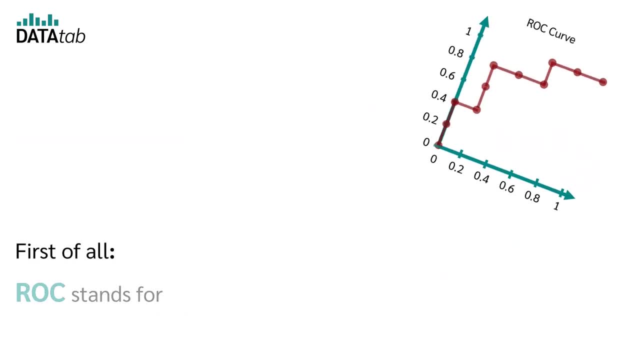 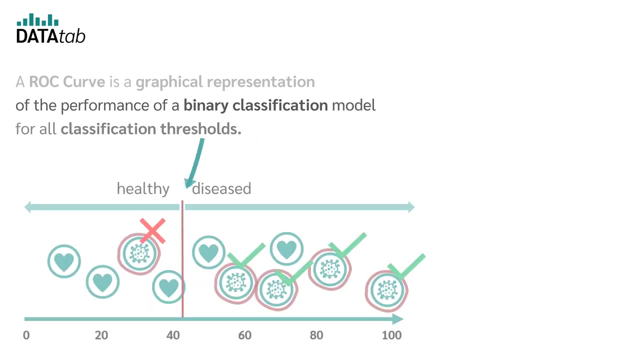 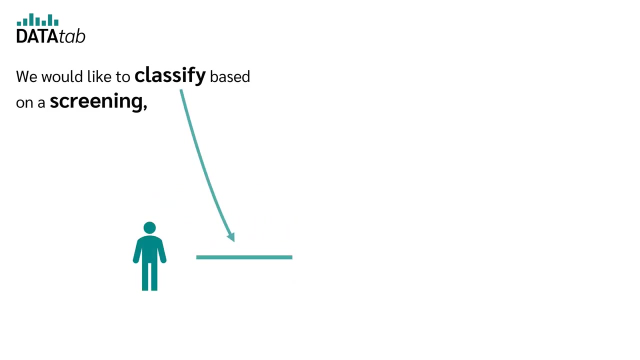 What is a ROC curve? First of all, ROC stands for Receiver Operating Characteristic. But what is a ROC curve? A ROC curve is a graphical representation of the performance of a binary classification model for all classification thresholds. Let's look at this with an example. We would like to classify, based on a screening, whether a person has cancer. 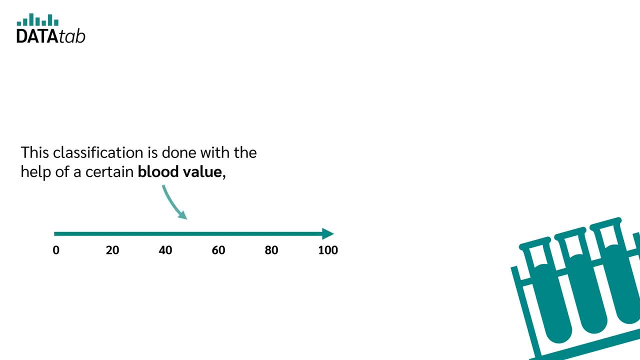 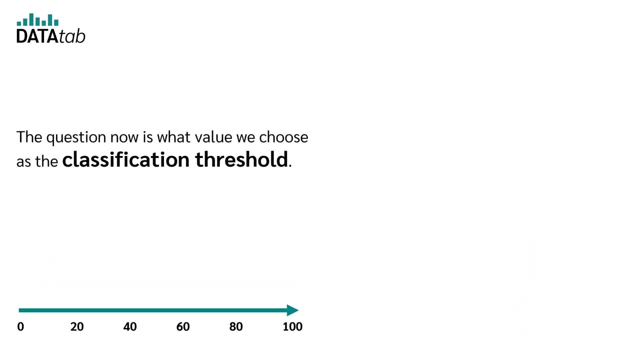 or not. This classification is done with the help of a certain blood value, where high values indicate cancer. The question now is what value we choose as the classification threshold. So at what level do we predict a disease? For this, we get data from 10 people about. 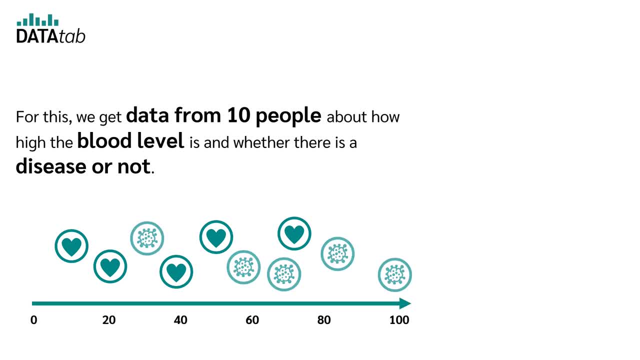